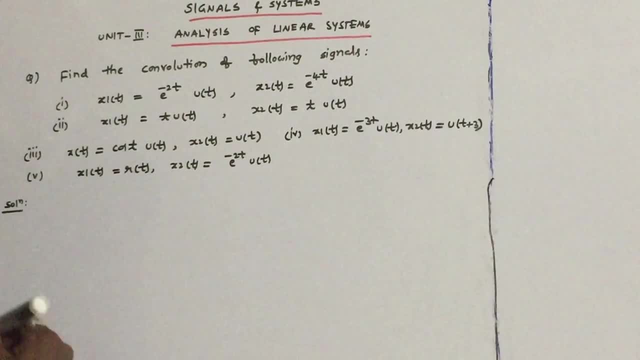 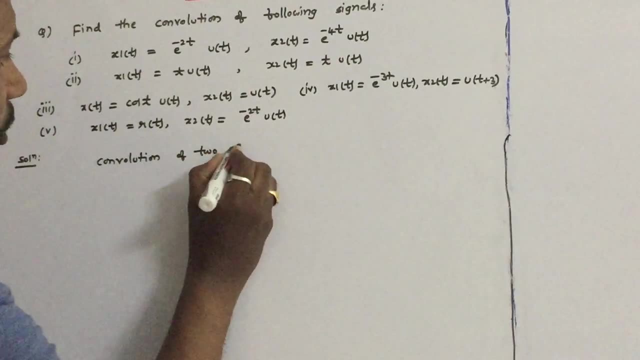 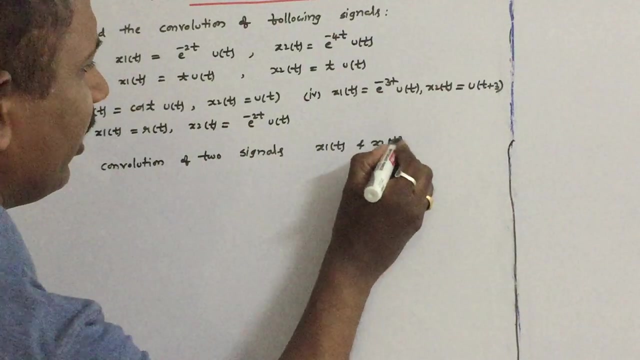 So, before going to do this problem, first let us write the convolution formula. The convolution of two signals, the convolution of two signals, x1 of t and x2 of t, is given by. is given by. first let us write the formula. 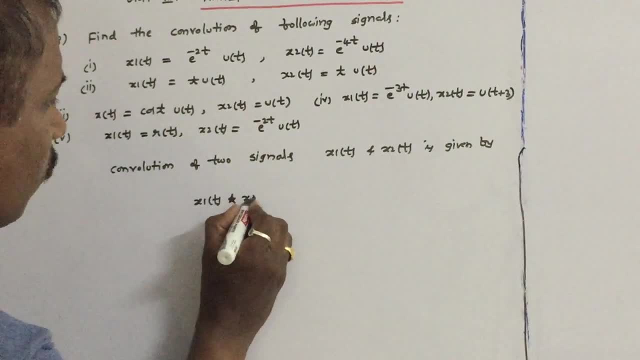 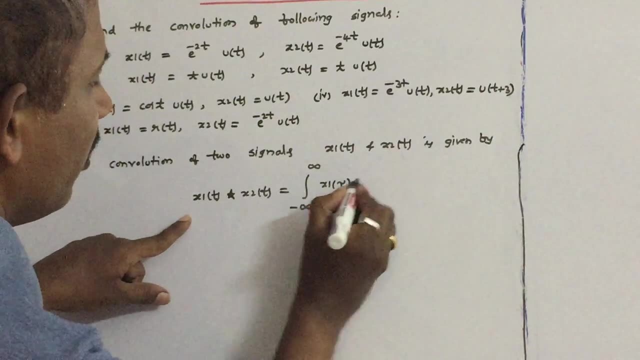 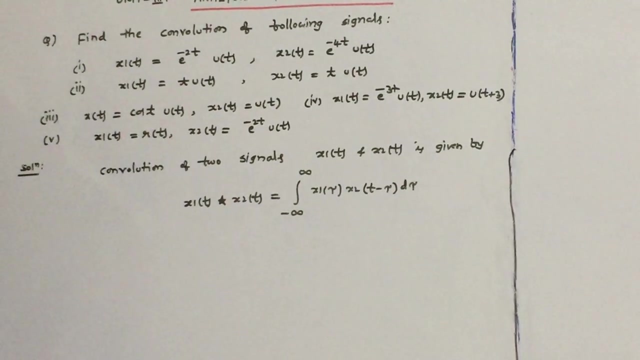 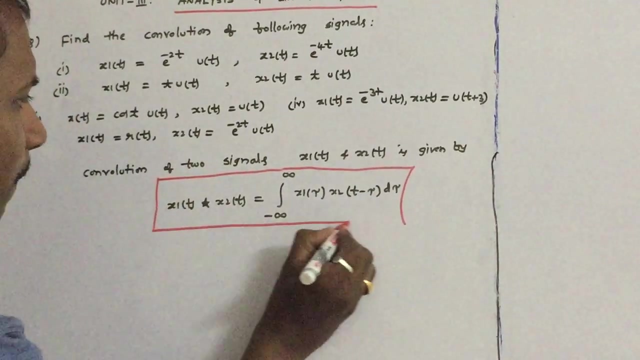 x1 of t, convolution with x2 of t is equal to integral minus. This is infinity to infinity. x1 of tau into x2 of t minus tau, d, tau. So I am going to use this formula to solve the given problems. So very, very important formula of this chapter. 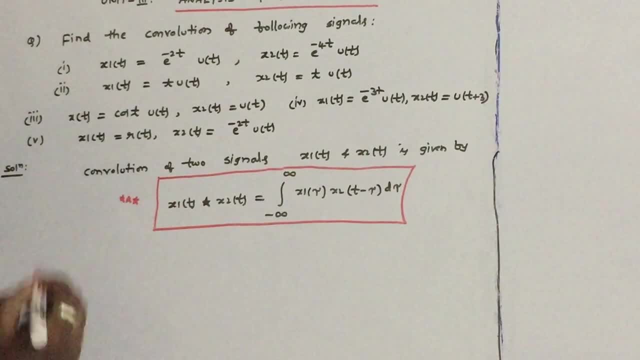 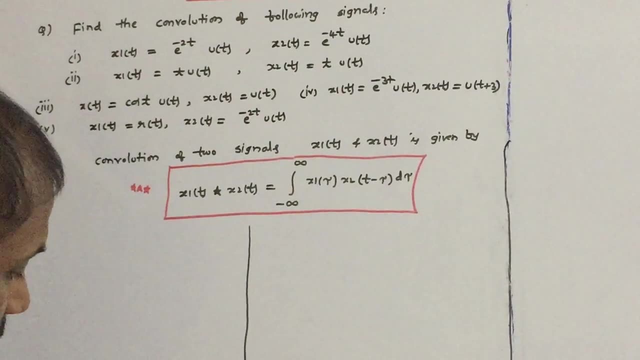 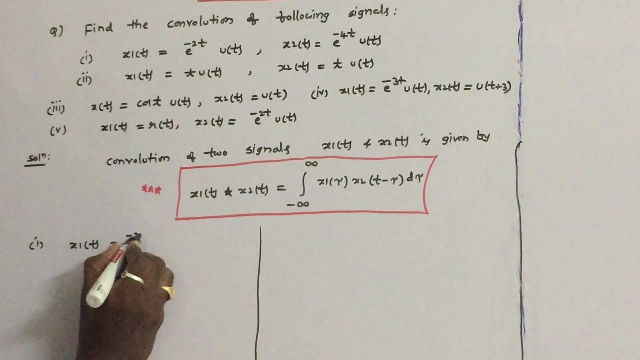 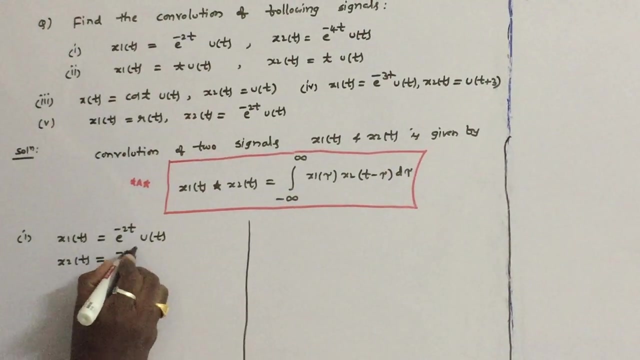 The convolution of two signals. So let us see the problems one by one. So number 1.. So what is the first problem given? What is x1 of t? x1 of t is given as e power minus 2 t into u of t. What is x2 of t is given as e power minus 4 t into u of t. 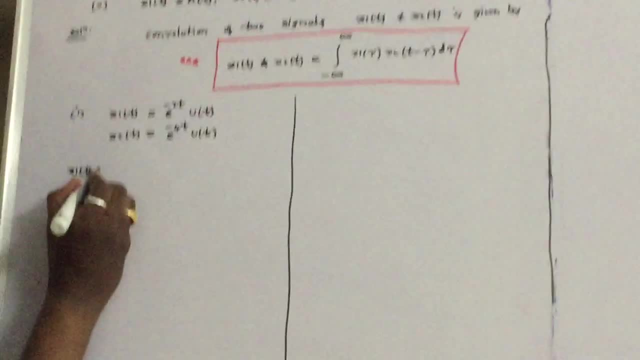 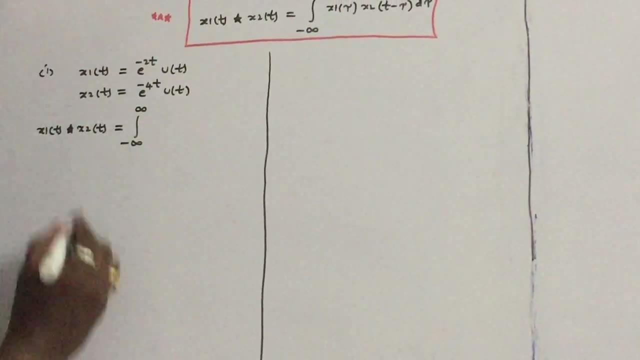 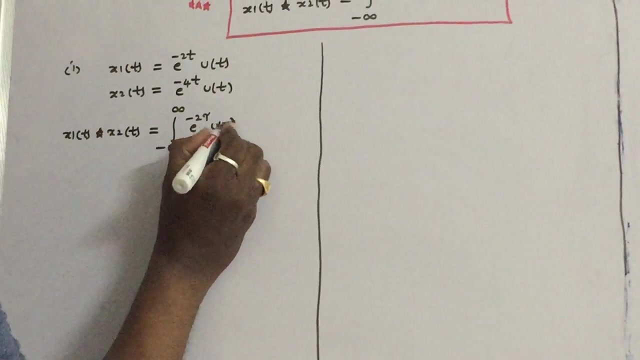 So first let us find out the convolution of these two x1 of t, convolution with x2 of t. formula integral minus infinity to infinity. First substitute in x1 of t, x1 of tau: power minus 2 tau into u of tau. x2 of t minus tau will become e power minus 4 into t minus. 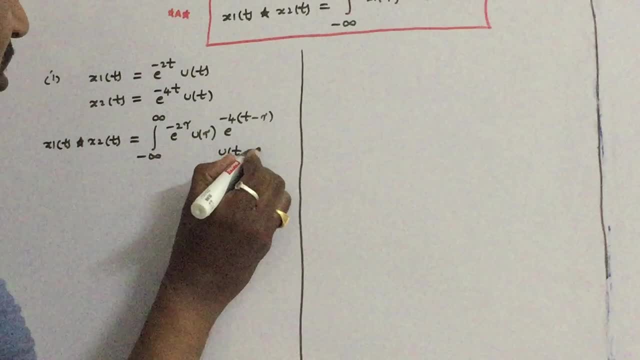 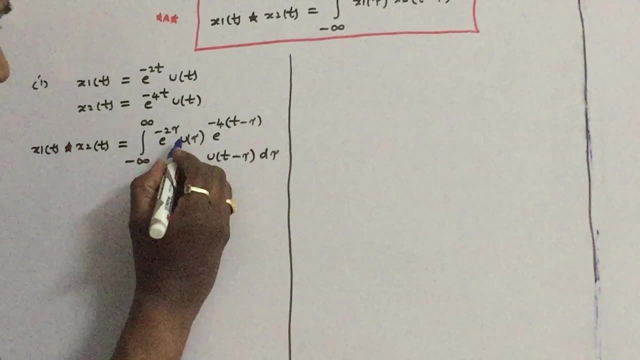 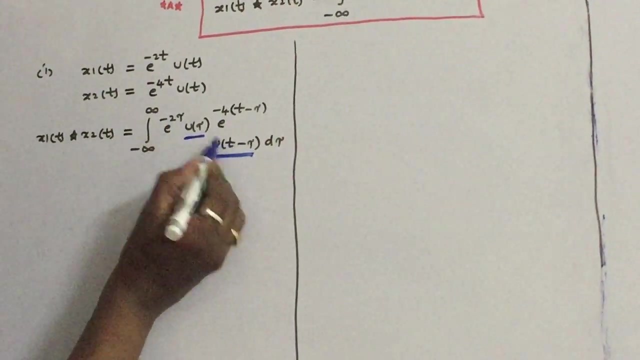 tau into u of t minus tau, d tau. so first let us write this. so here this multiplication is very, very important: u of tau and u of t minus tau. so therefore the limits will change because of this: u of tau and u of t minus tau. let us see this integration is with respect. 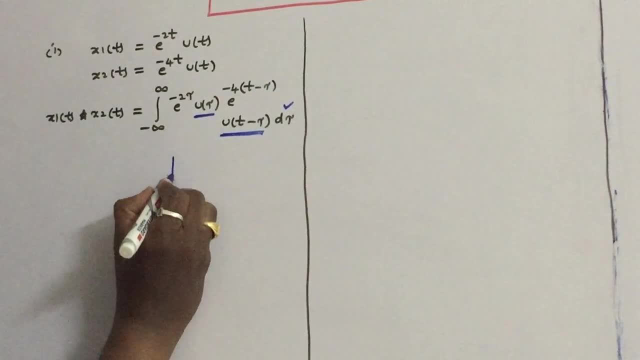 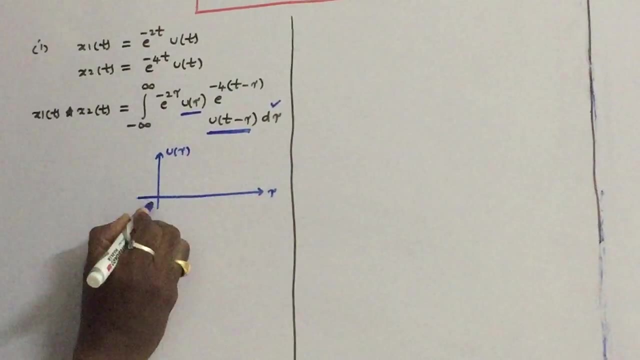 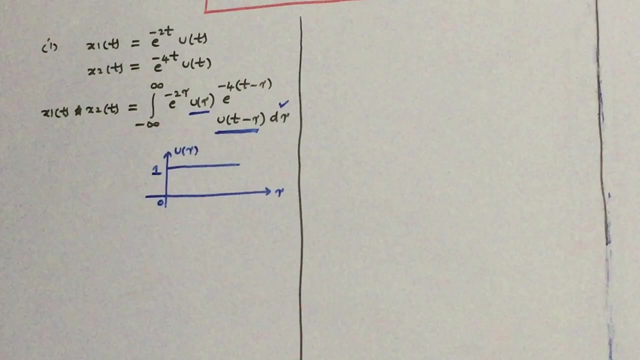 to tau. remember that first let us write u of tau. so what is u of tau? nature u of tau graph is u of versus tau. so the graph of u of tau will be 1 from 0 onwards. so let us plot u of u of u of. you can see that u of tau is 1 from 0, so let us plot u of u of u. 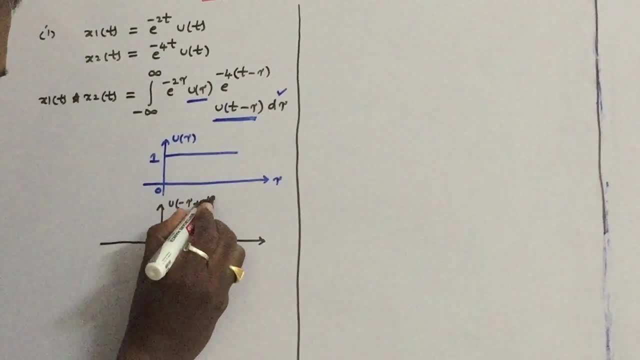 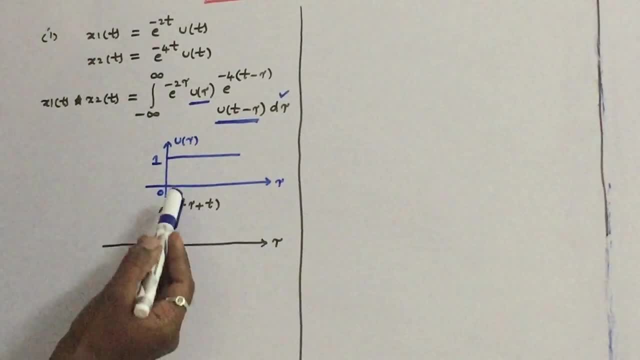 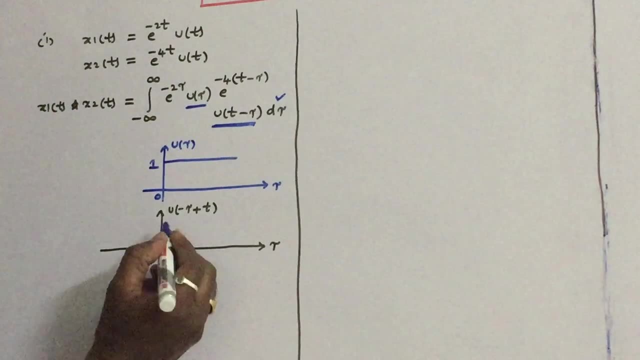 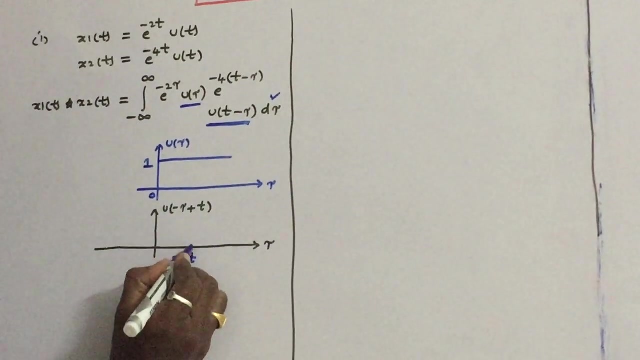 because this is tau's axis. so where this is time-reversed unit step signal, so therefore we have to draw left side the time-reversed unit step signal. but where this step starts at, tau is equal to t, so therefore this step starts Here, tau is equal to t, is equal to t, so 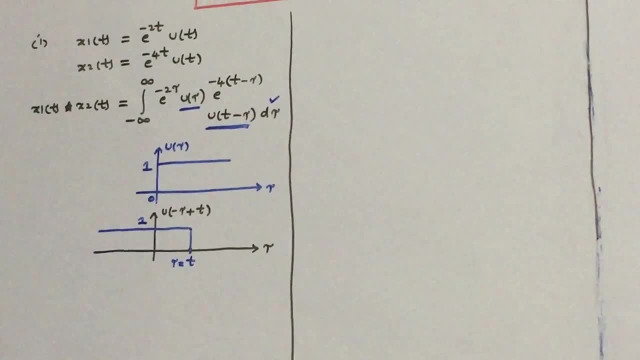 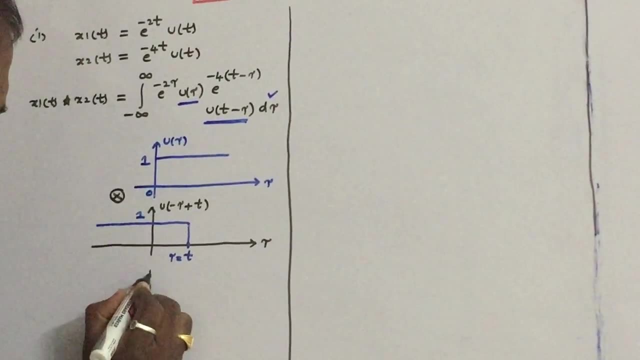 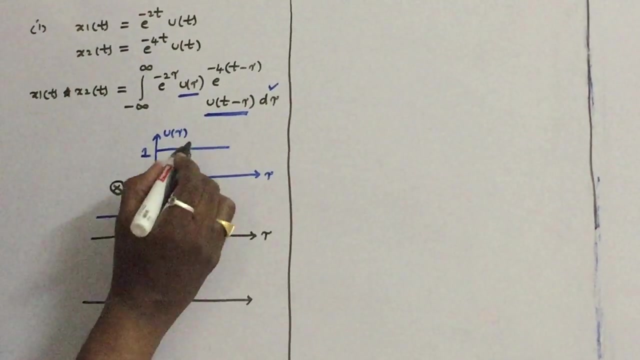 t will be towards the Left side of amplitude 1. you can see that if you multiply two tangential this, u of tau and u of t minus tau, very, very important. so therefore you can see that, you can see that. so if you multiply this, so this portion is zero. so this portion is zero only. 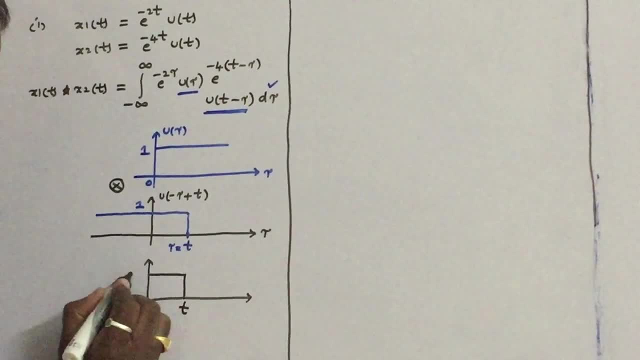 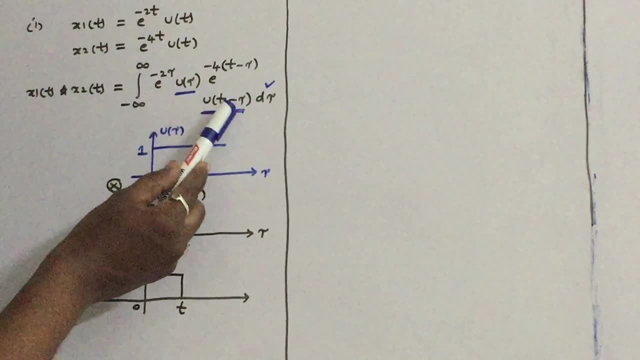 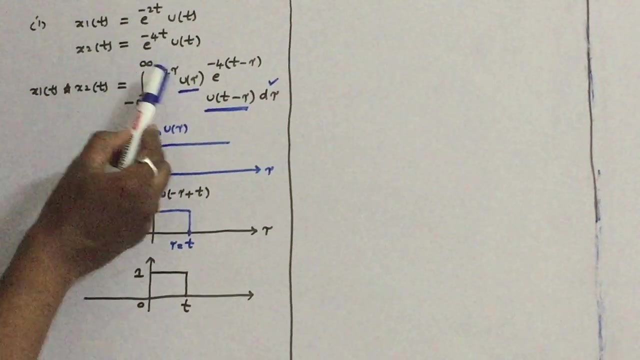 the pulse will remain from zero to t, of amplitude one. so therefore remember in this problem. so therefore, so, when u of tau is multiplied by u of tau, t minus tau, so the limits will change from zero to t. zero to t in the general u of tau amplitude is one, u of t minus tau. 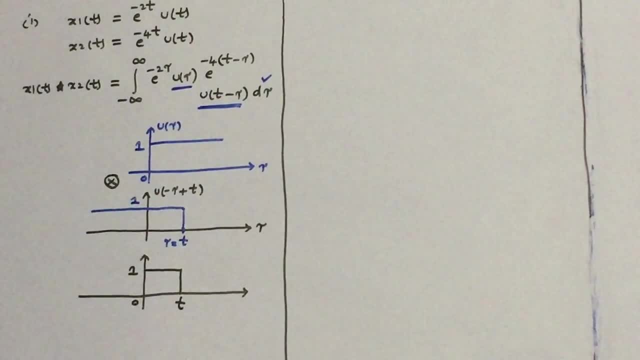 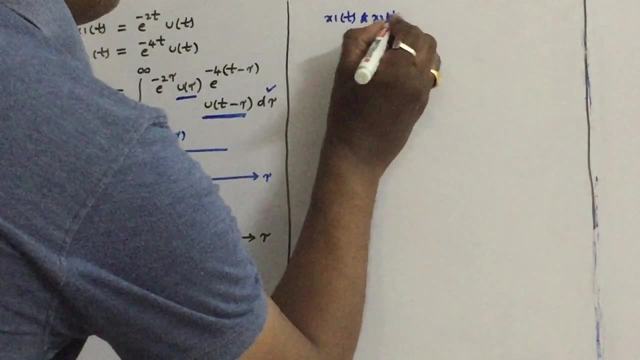 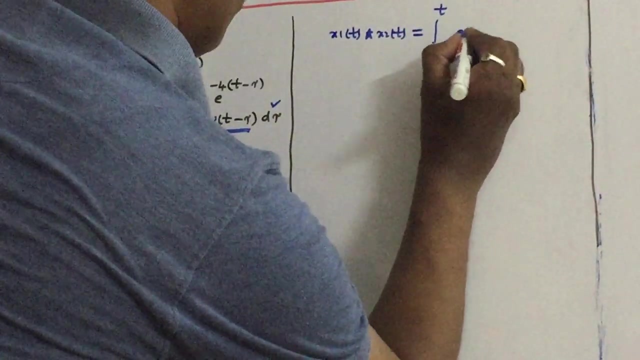 amplitude is one, one into one is one. so therefore, that is one very, very important point in this problem. so therefore, x1 of tau converges with x2 of tau, so that is equal to what i am writing. i am changing the limits from zero to t, so e power minus 2 tau. e power minus 2 tau into. 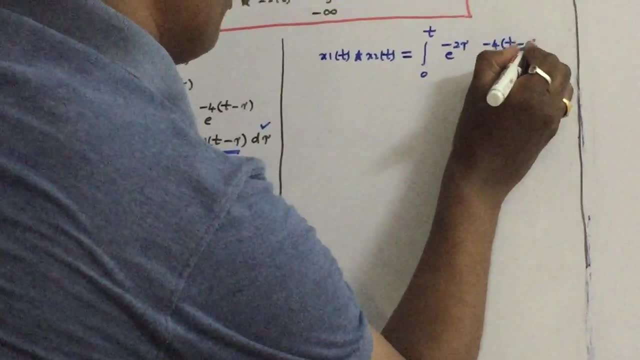 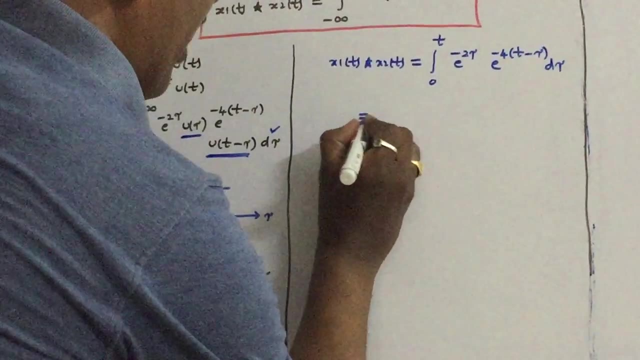 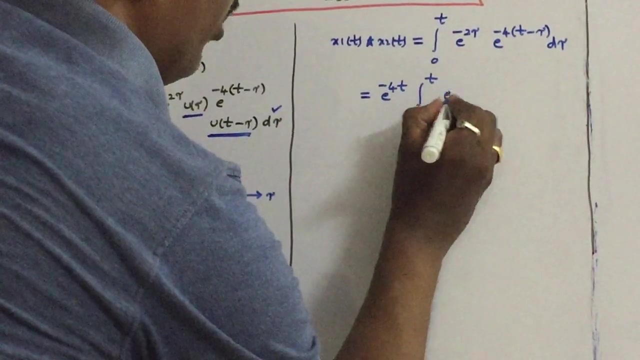 e power of minus 4 into t minus tau d tau. so what is the constant? because this integration with respect to tau e power minus 4 t is a constant. you can take it outside integral zero to t e power 4 tau minus e power 2 tau, it will become e power 2 tau d tau. so you can check that e power. 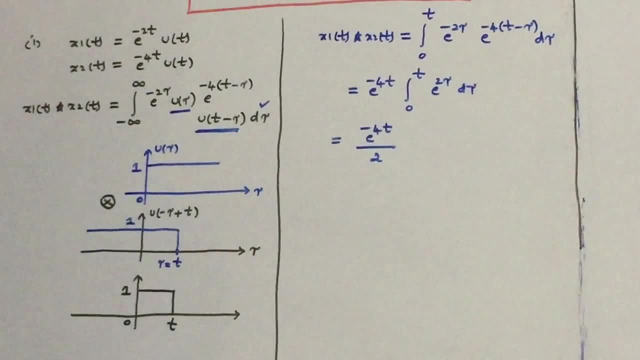 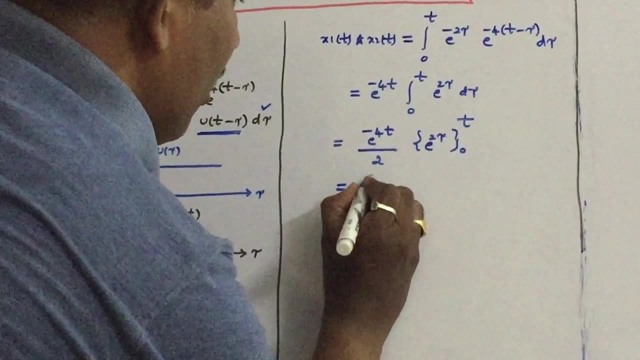 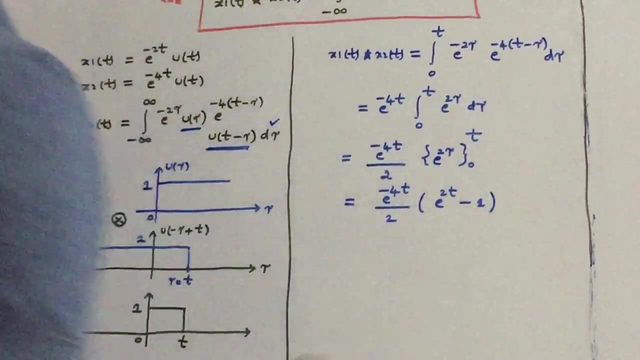 minus 4 t by integration is e power 2 tau by 2, so therefore e power 2 tau substitute the limits zero to t. so e power minus 4 t by 2 into e power 2 t minus e power zero is 1. so if you multiply: 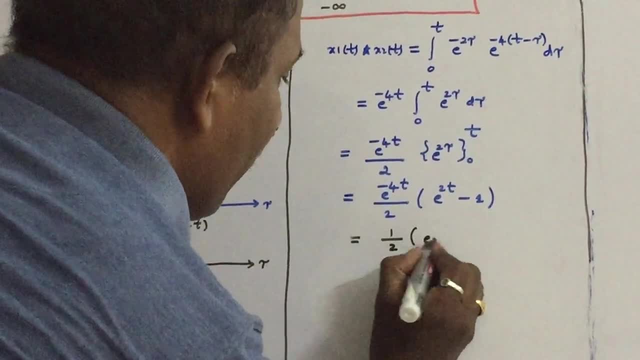 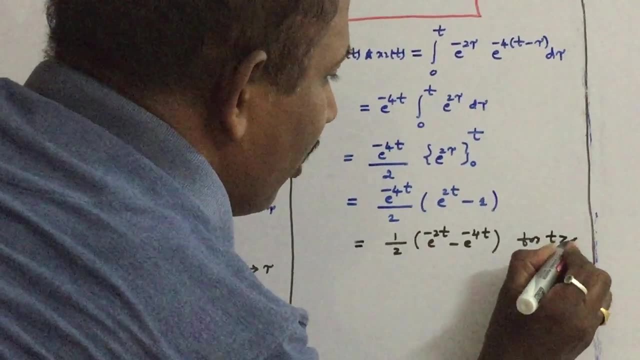 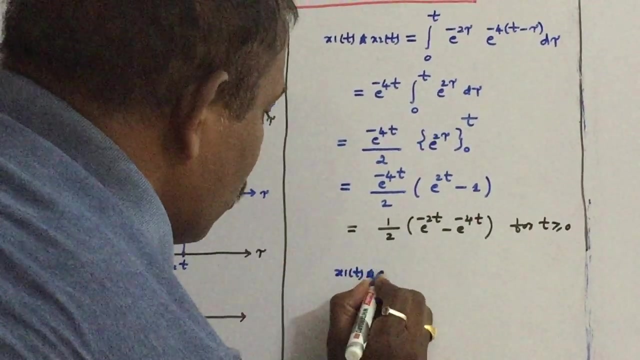 this. the answer is 1 by 2 into e power minus 2 t minus e power minus 4 t. we have to clearly write: for t greater than or equal to zero. this answer is for t greater than or equal to zero, or otherwise: x1 of t convolution with the x2 of t answer is also equal to 0, that is. 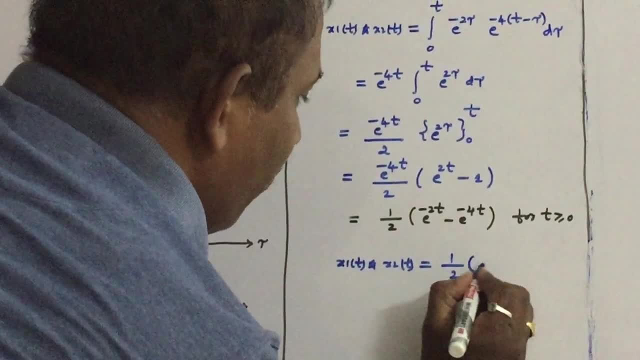 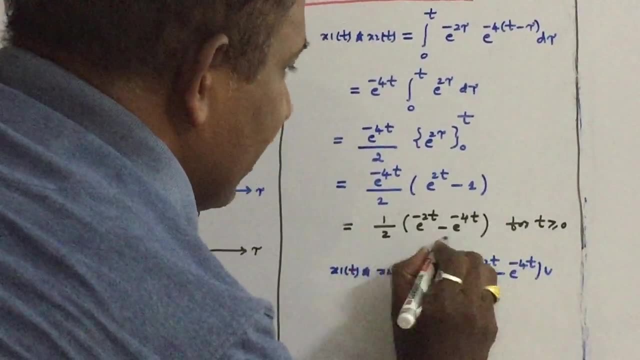 very important, written as 1 by 2: into e power minus 2t minus e power minus 4t. into you have to add, because this signal you have to take from t greater than or equal to 0, just add u of t, so this: 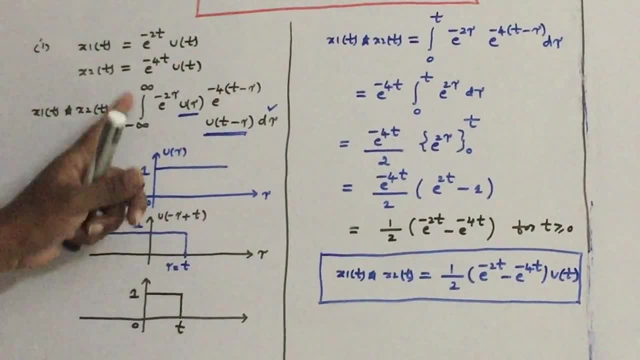 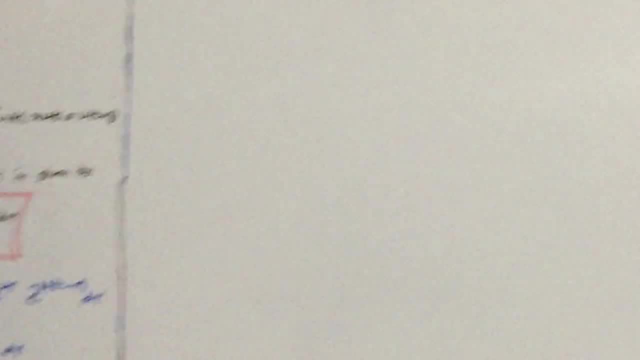 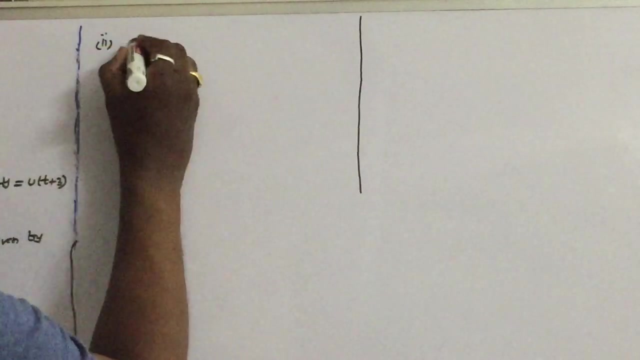 is the answer for the first one. the important point is changing the limits of integration. now let us see the in similar manner. the second problem, the second problem, the second problem. what is the second problem given? the second problem is given as x1 of t. x1 of t is equal. 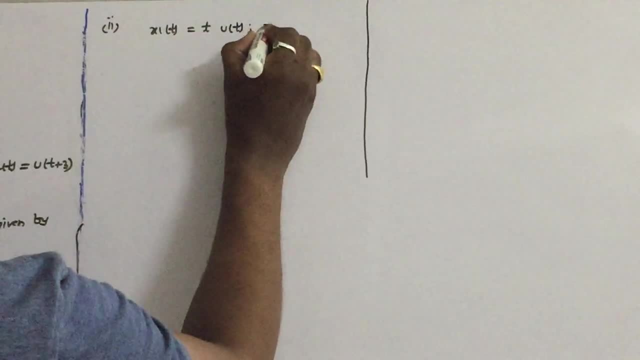 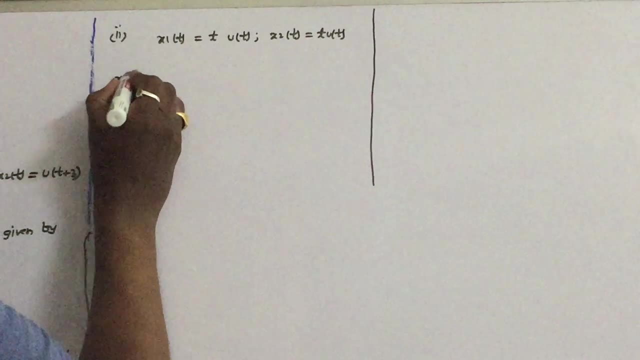 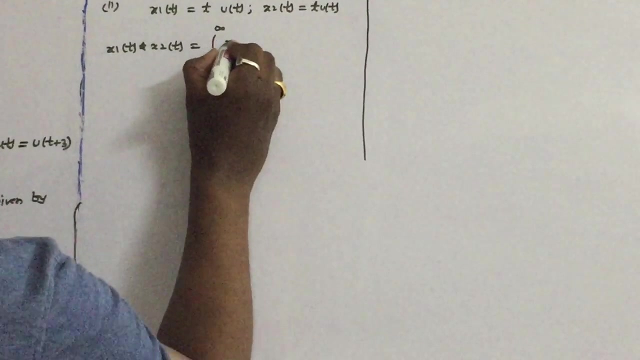 to t into u of t, and x2 of t is also equal to t into u of t. first let us write the formula. the convolution of two signals, x1 of t into x2 of t, is mathematical, and x2 of t is also mathematically defined as integral minus infinity to infinity. x1 of tau into x2 of. 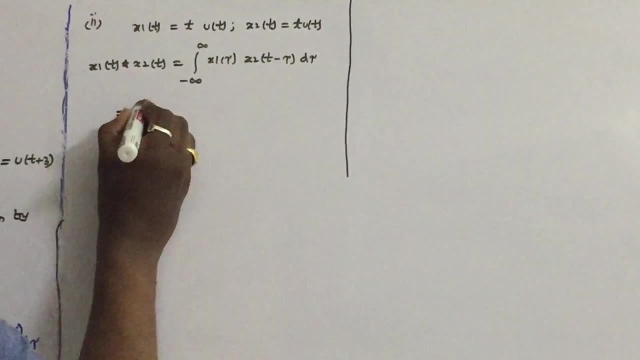 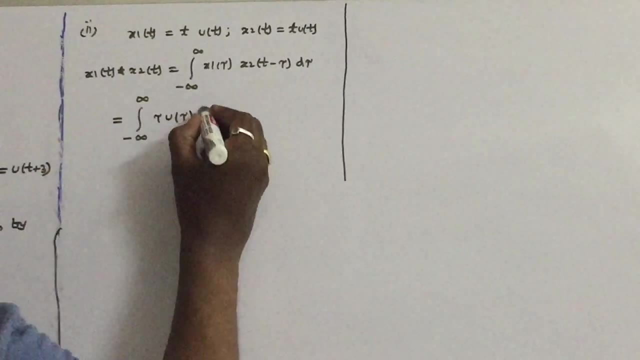 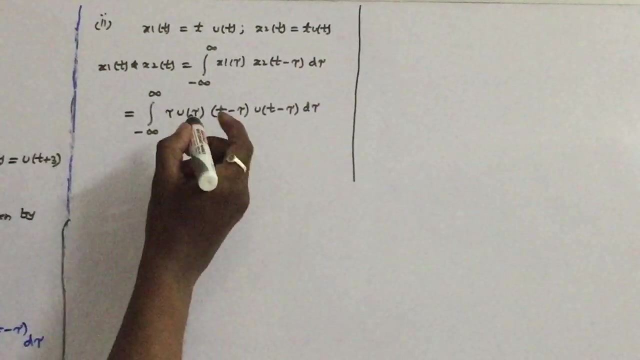 t minus tau d tau. so let us just let us substitute the limits. if x1 of tau, what is x1 of tau, will become tau into u of tau. x2 of t minus tau will become t minus tau into u of t minus tau d tau. so you can see that, because of this u of tau and u of t minus tau, multiplication. 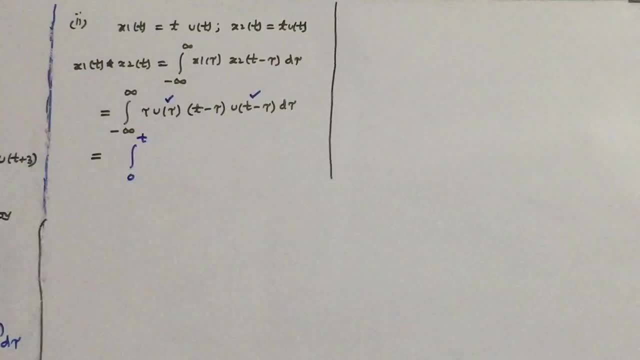 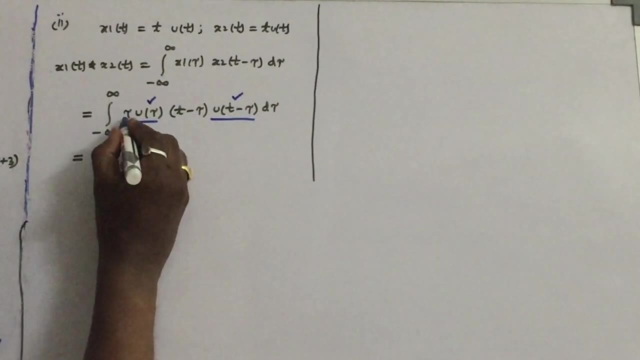 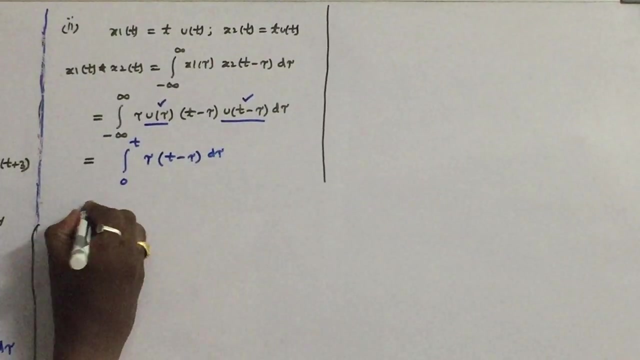 you can change the limits. in the previous problem we have seen we have to change the limits from 0 to t in this interval. its amplitude is 1, its amplitude is 1, 1 into 1 is 1. so therefore, what is the remaining part? tau into t, minus tau, d, tau, d tau. just take the tau inside integral. 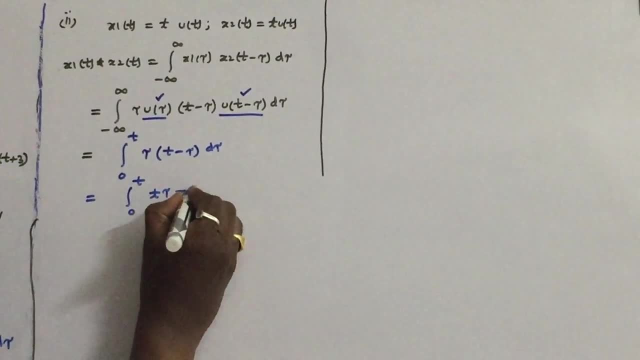 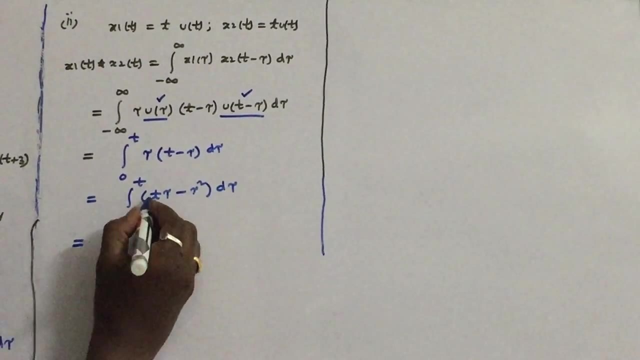 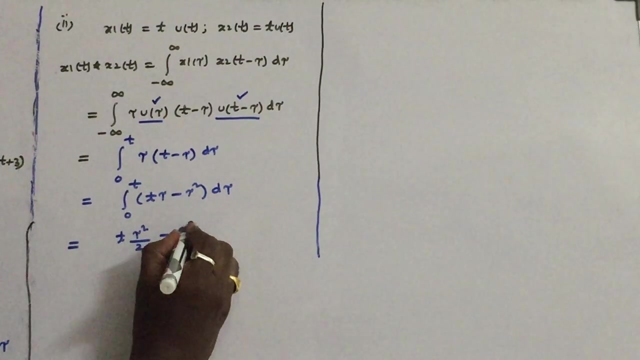 0 to t. t tau minus tau square into d tau, so d tau so. therefore you can take it as so. t is a constant. what is integration of tau? tau square by 2 minus integration of tau square? is tau cube by 3? just substitute the limits 0 to t. if you substitute the t in place of 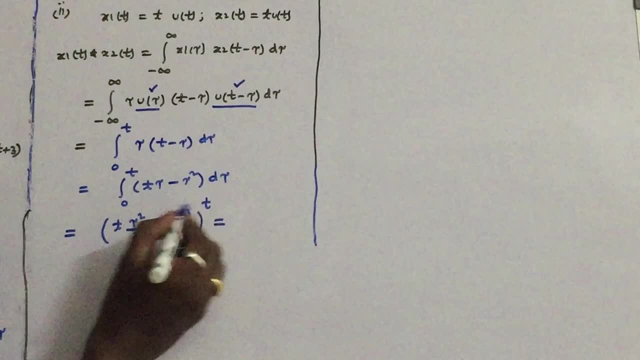 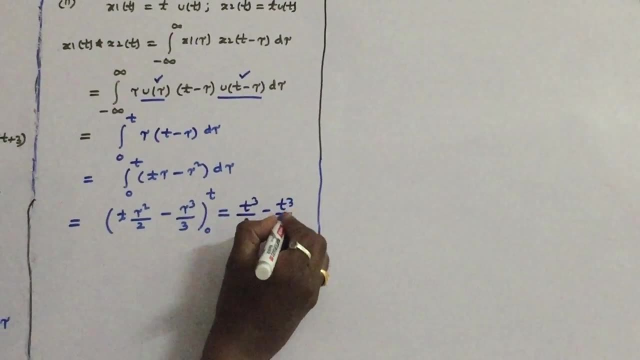 tau. tau square into tau. tau square t square, t square into t. it will become t cube by 2 minus t cube by 3. if you substitute the lower limit in place of tau 0, 0, the lower limit will become 0. it will become tau square into t 4 by 3. so this is the 표현: t square into. 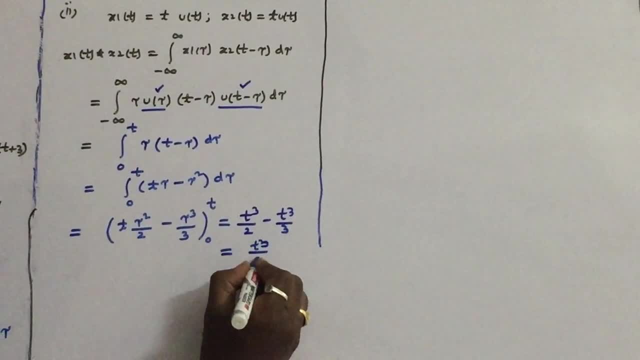 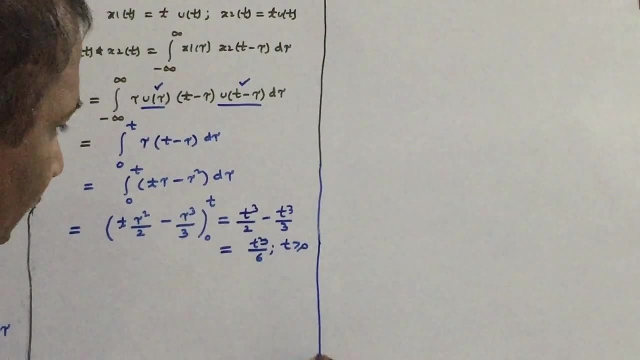 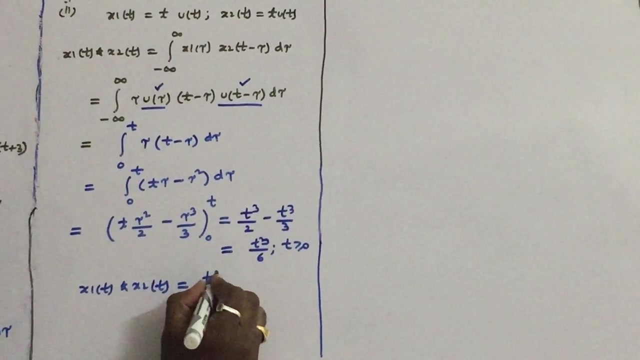 tau 1 by 3.. cube by 6 tau. cube by 6 for t greater than or equal to 0 or otherwise, you can write the same answer as so: x1 of t, convolution with x2 of t, is written as t cube by 6 into u of. 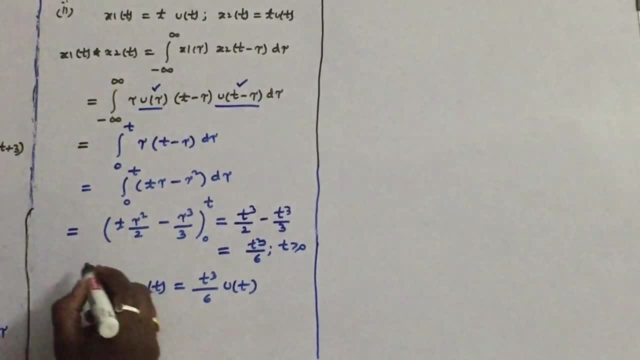 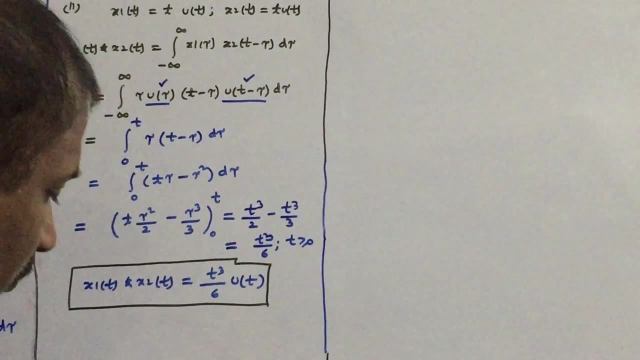 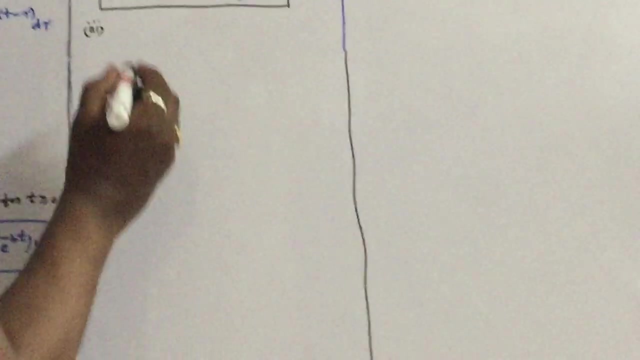 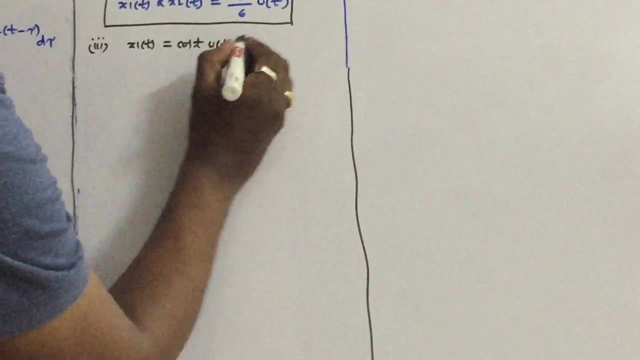 t. so this is answer for the 2nd problem. this is the answer for the 2nd problem, so let us see the 3rd problem. so what is it given? x1 of t is given as cos t into u of t and x2 of t is given as u of t. they must take: 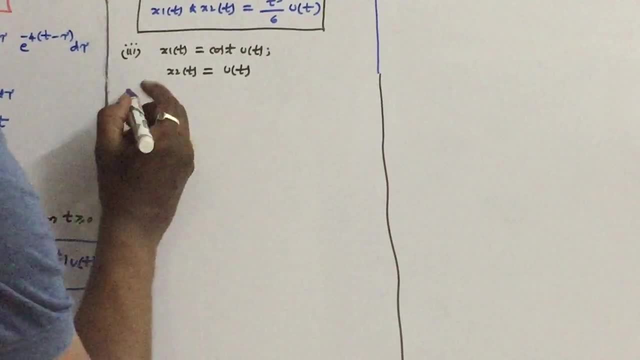 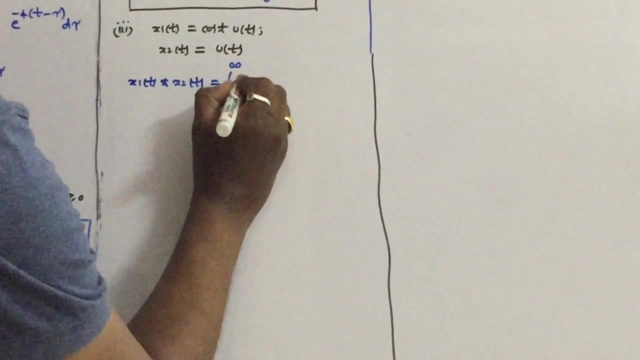 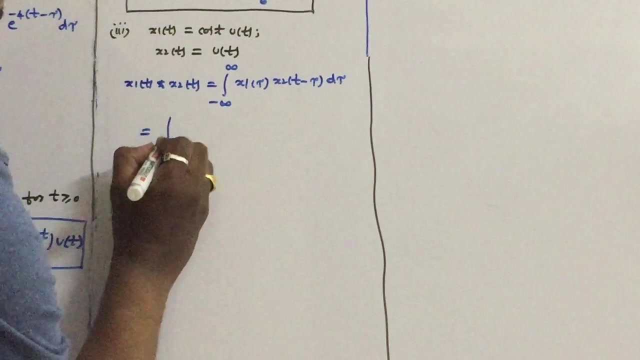 those terms carefully. So let us write the first formula. So what is x1 of t, convolution with x2 of t? Just write the formula Integral minus infinity to infinity, x1 of tau into x2 of t minus tau d tau. So first just substitute integral minus infinity to infinity. 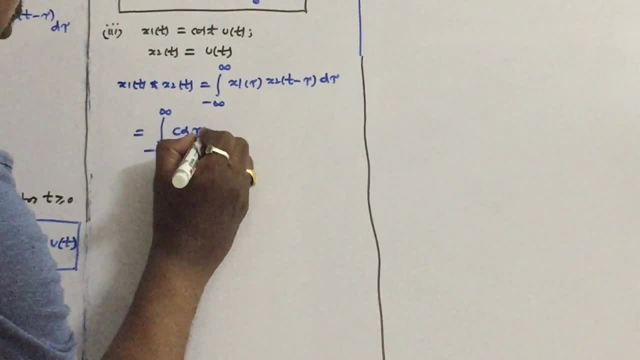 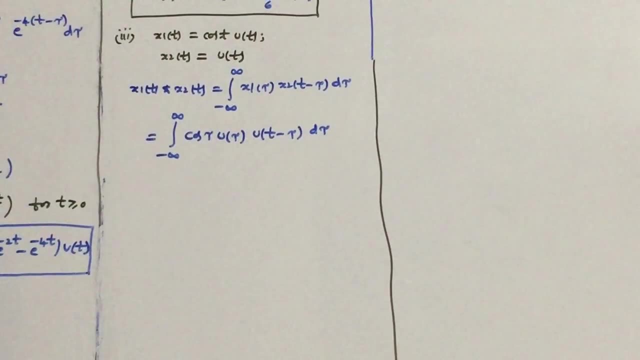 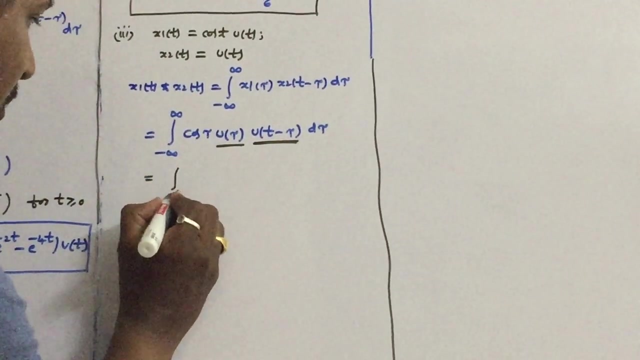 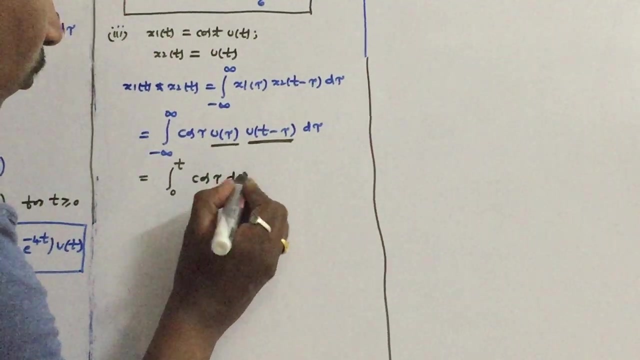 What is x1 of tau. Cast tau into u of tau. What is x2 of t minus tau, u of t minus tau d tau. So if you multiply both of them, as we discussed previously, change the limits from 0 to t In this interval. this multiplication answer is 1.. So therefore, cast tau d tau. 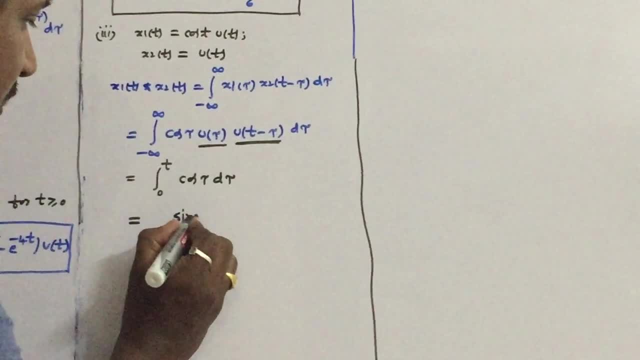 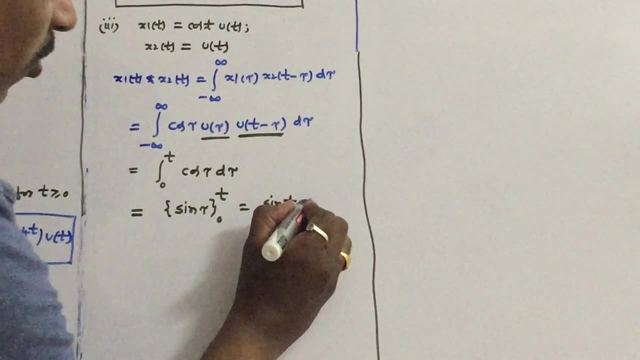 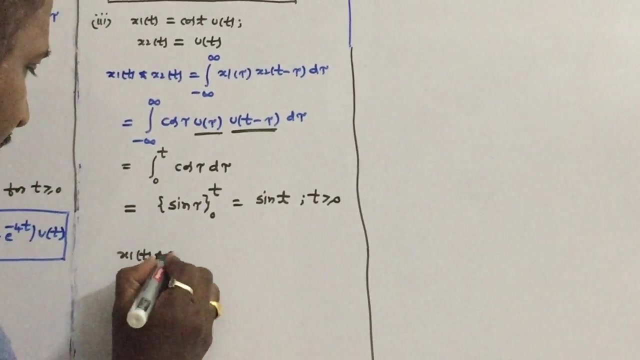 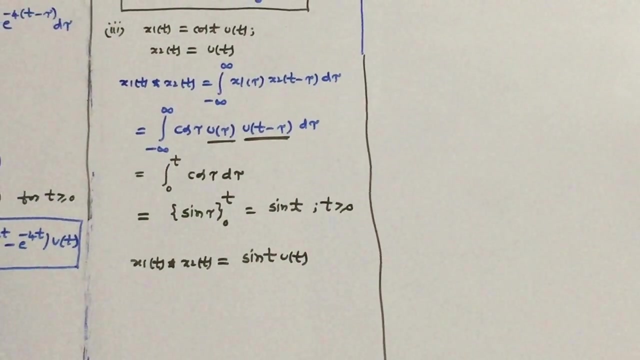 So what is integration of cast tau, Sine tau, Sine tau. So if you substitute the limits 0 to t, so it will come out as sine t. Sine 0 is 0. So this is for t greater than or equal to 0. Otherwise you can write the same answer as x1 of t, convolution with x2 of t, answer as sine t into u of t. So this is the answer for this problem: Convolution of two given signals. 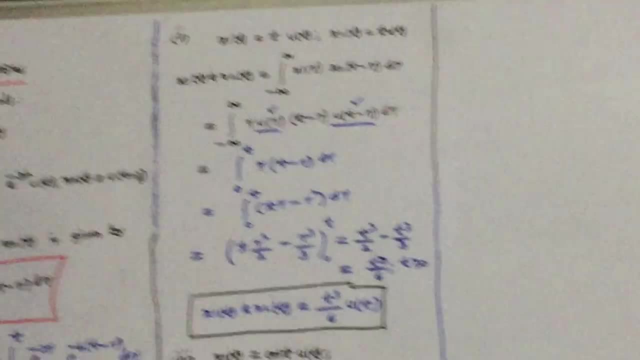 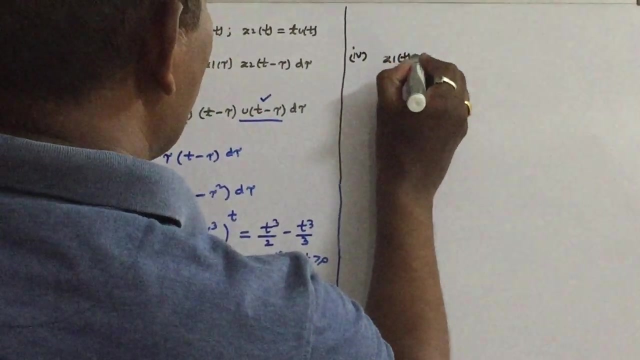 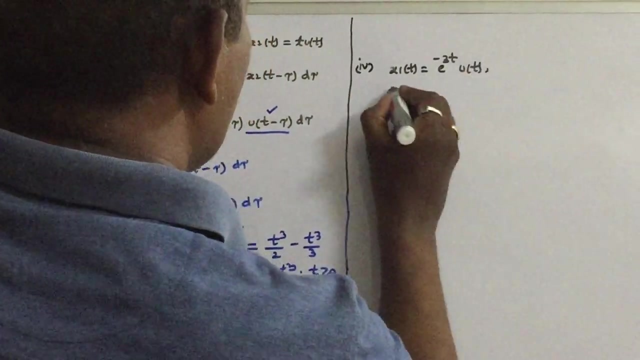 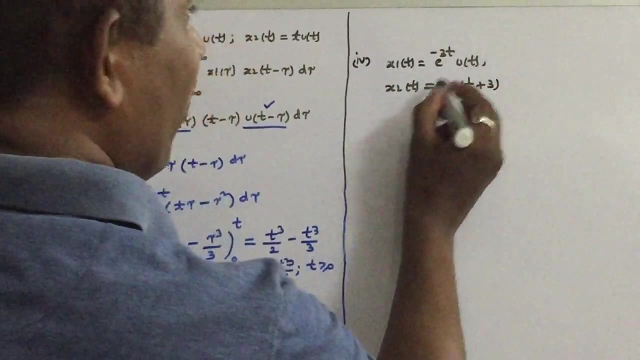 So let us take the fourth problem. The fourth problem is: x1 of t is equal to e power minus 3t into u of t, and x2 of t is equal to u of t plus 3.. See for the two signals. you observe that u of t, this one, this is not u of t. 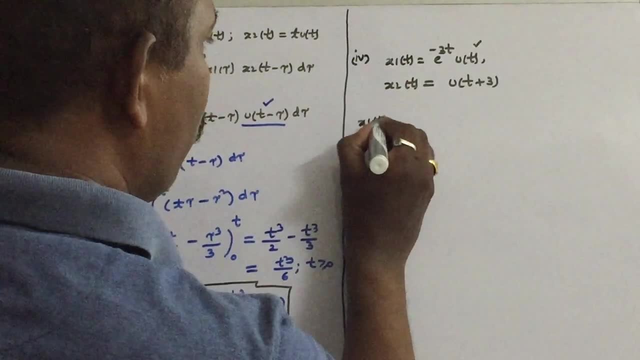 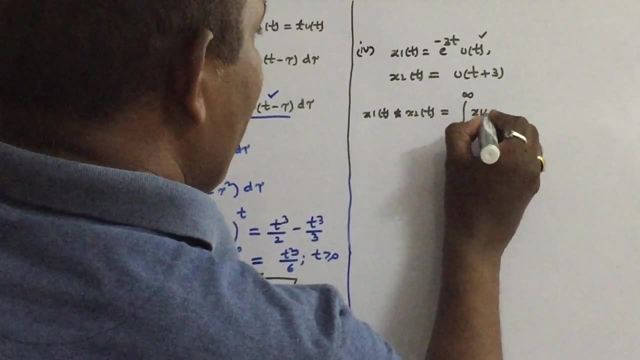 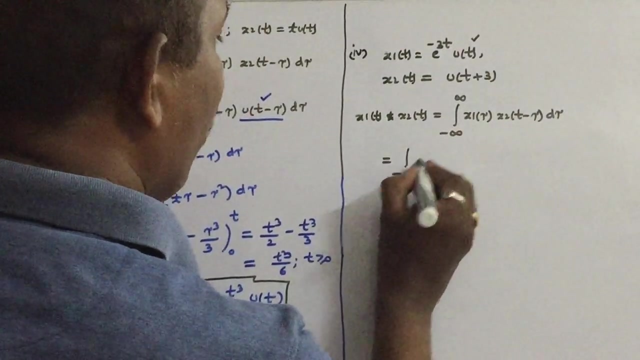 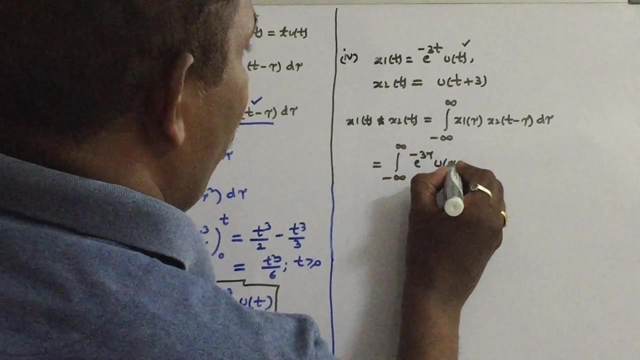 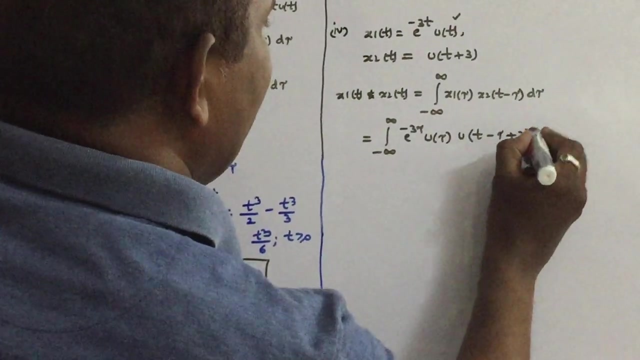 So therefore, first let us write the formula. what we have to do? x1 of t- convolution with x2 of t is equal to first write the formula: integral minus infinity to infinity. x1 of tau into x2 of t minus tau d tau. First let us substitute x1 of tau and x2 of t minus tau. Integral minus infinity to infinity. x1 of tau is e power minus 3 tau into u of tau. x2 of t minus tau is you clearly check that u of t minus tau plus 3 d tau. 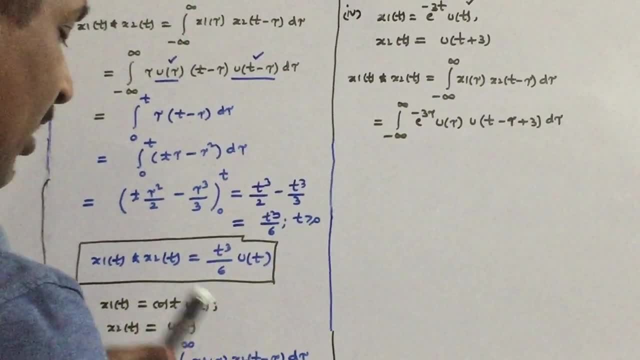 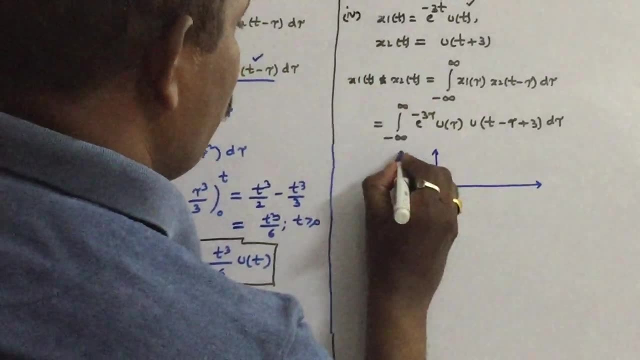 So we have to hear carefully, we have to change the limits. So first, for this purpose, first let us draw u of tau. First let us draw u of tau. So this is u of tau versus tau. Its amplitude is 1.. 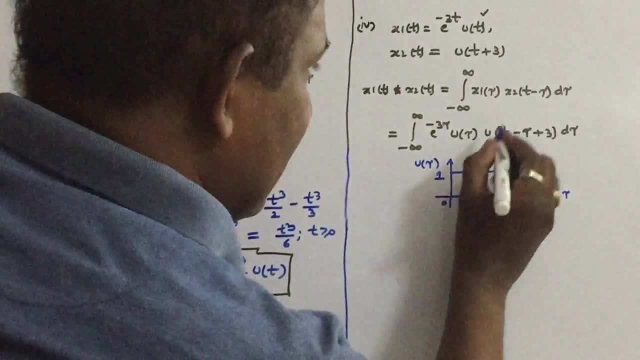 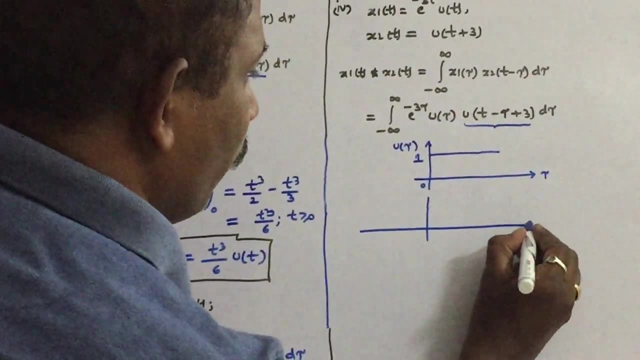 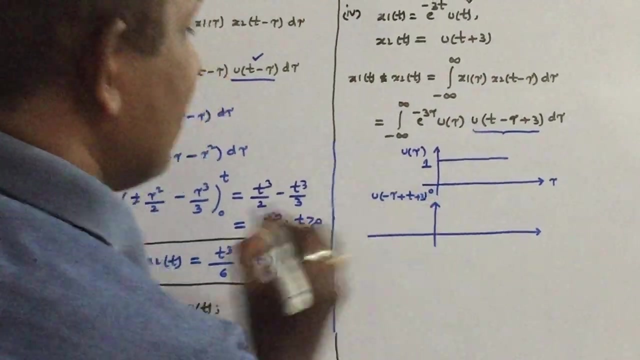 Its amplitude is 1.. So this is the second one, This one. how to draw this? How to draw this? What is this? u of Minus tau tau plus t plus 3.. So, where it is starting, Minus tau plus t plus 3 is equal to 0. So 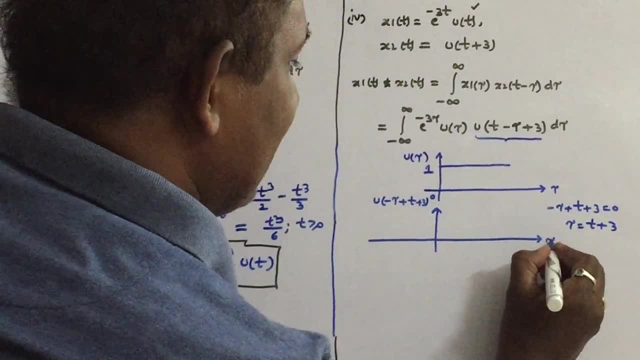 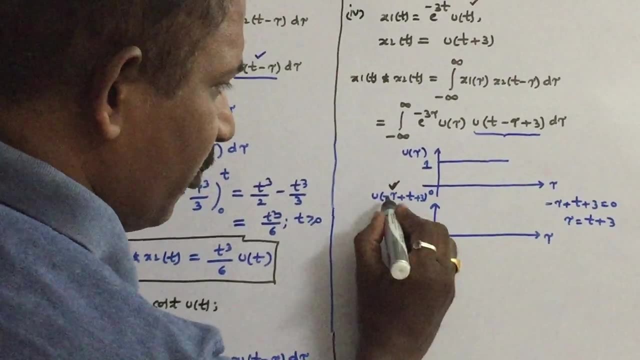 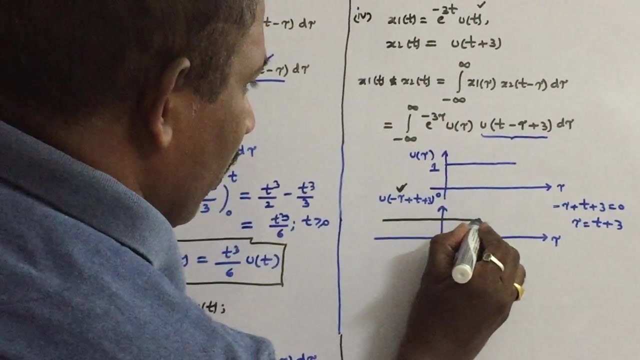 that is, tau is equal to t plus 3.. So remember that this axis is tau. So therefore, so, since this is a time reverse linear step, where this linear step is starting At t plus 3, remember t plus 3 towards left side, If you multiply both of them, if you multiply both, 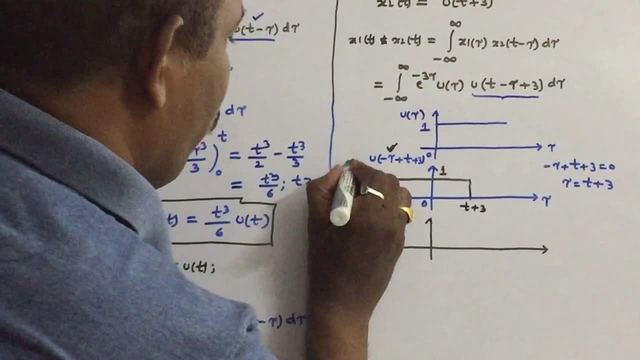 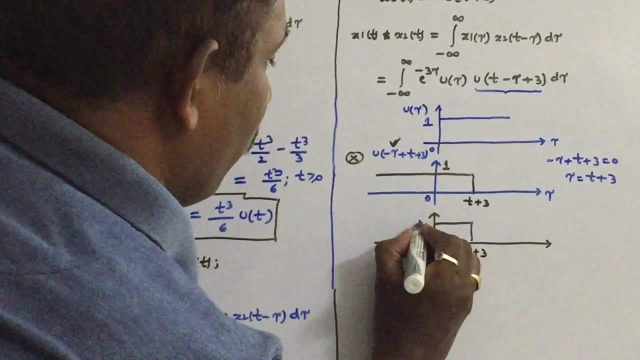 of them, if you multiply both of them. so what is the answer of the pulse? So it is existing from 0 to t plus 3 of amplitude 1.. So this is the important point we have to note. So, therefore, so because this multiplication, in this multiplication, change the limits. 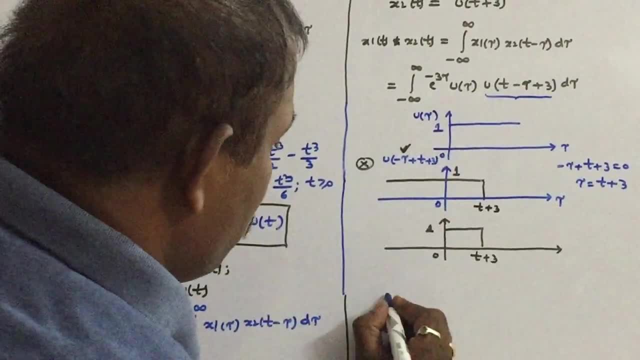 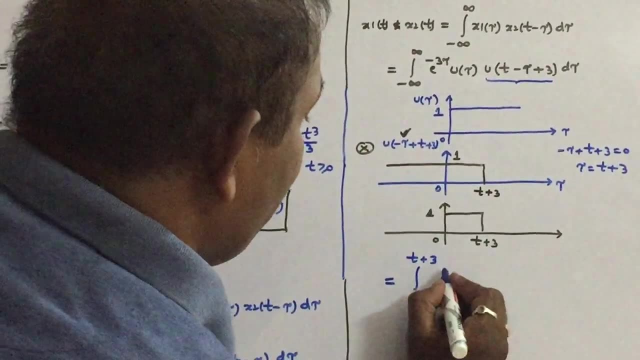 from 0 to t plus 3.. So that is the only substitution we are making. So therefore, instead of 0 to t plus 3, it is not t remember that in this problem. So therefore, e power minus 3, tau d tau. So what? 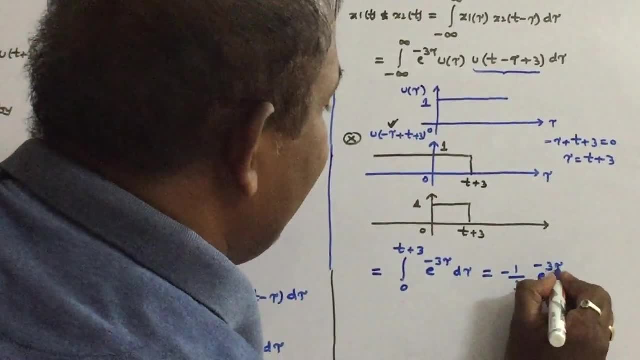 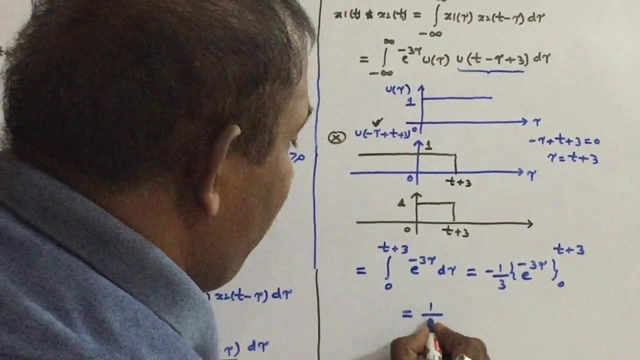 is the integration Minus 1 by 3 into e power minus 3 tau. substitute the limits 0 to t plus 3.. If you substitute, the answer will come at upper limit and lower limit. multiply minus sign, So it will come out as 1 minus e power. 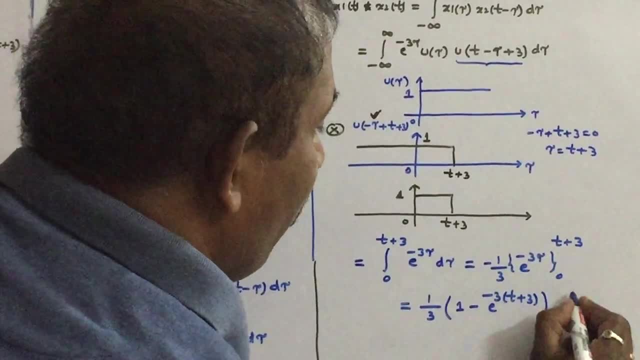 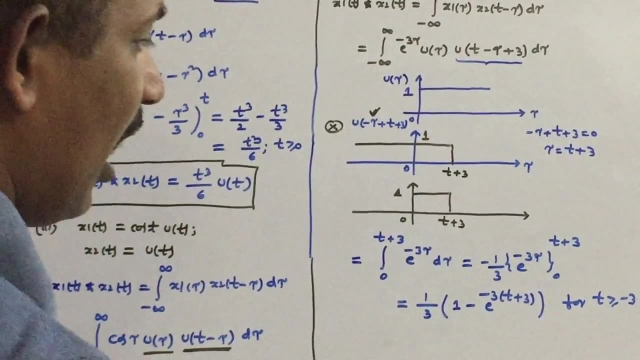 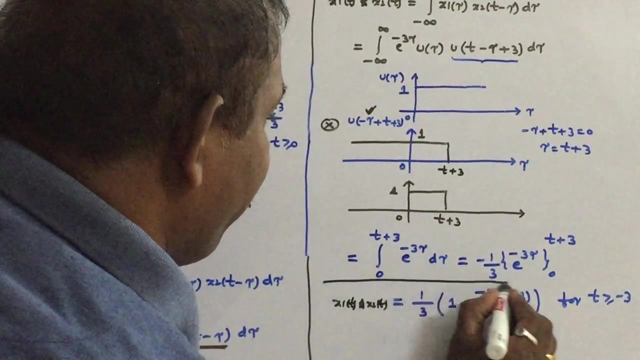 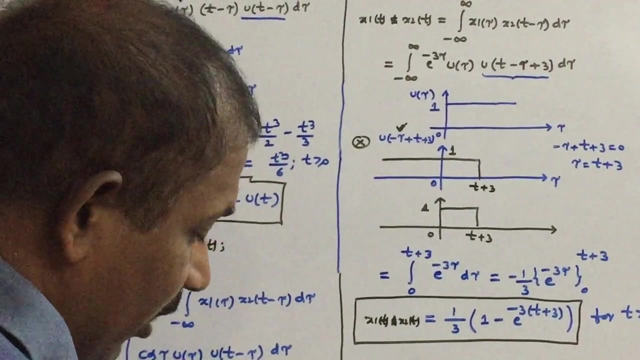 So is equal to minus 3 into t plus 3.. We have to earlier write, for this signal is from t greater than or equal to minus 3.. So this is the answer for this problem. x1 of t is convolution with x2 of t the answer for this problem. So let us do the last problem. let 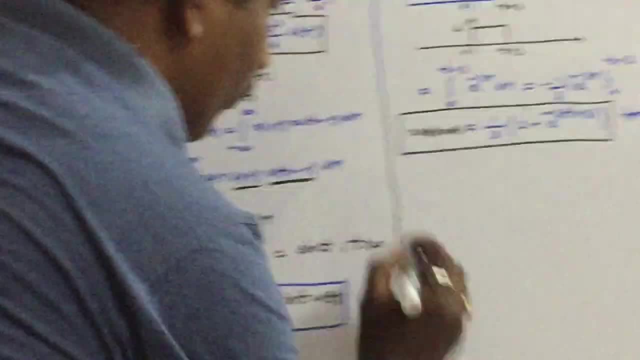 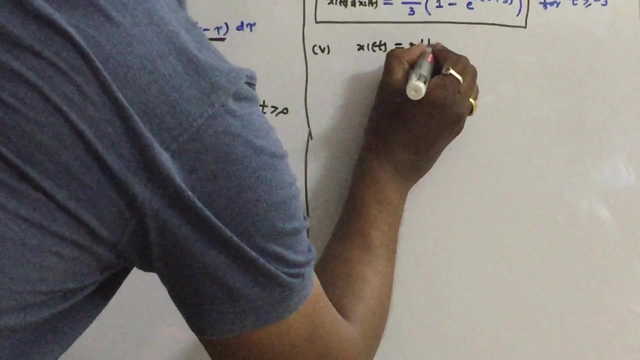 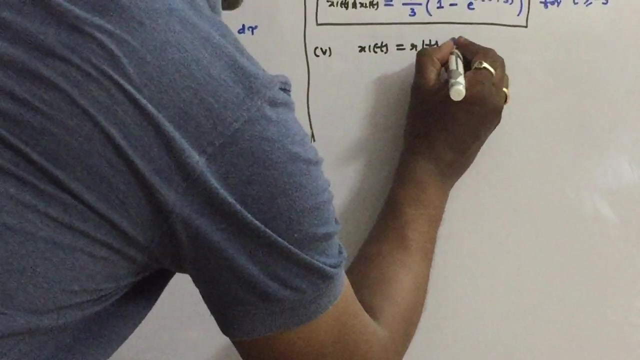 us do the last problem, fifth one. Fifth one: What is x1 of t is given. x1 of t is given as r of t. r of t means ramp. So you have to observe this is a ramp unit, step ramp. So we can also write this as t into u of t. 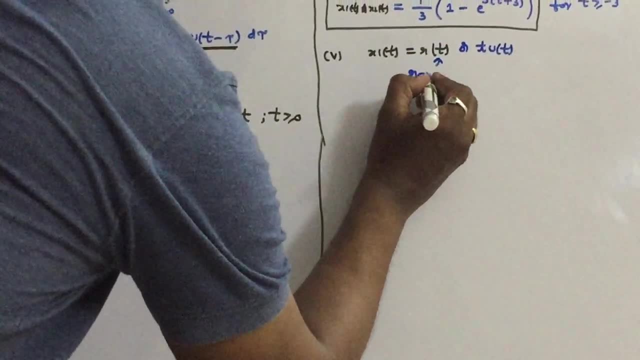 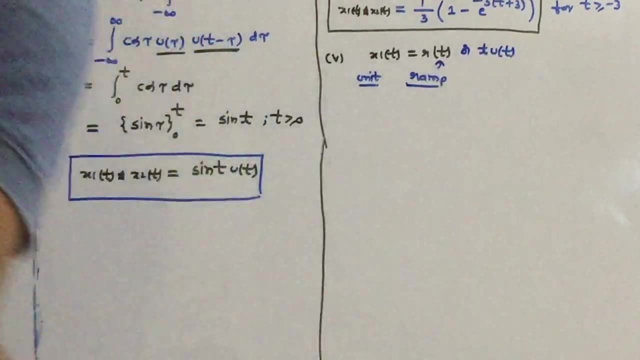 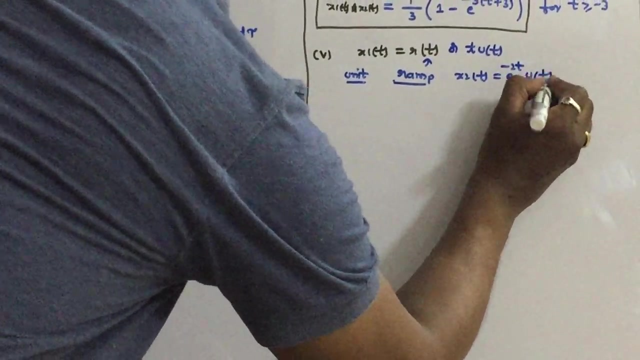 So you have to, also because it is a ramp unit, step ramp, unit ramp. So unit ramp means its slope is 1.. So therefore you can write like this: So what is x2 of t? So x2 of t is equal to e power minus 2t into u of t. 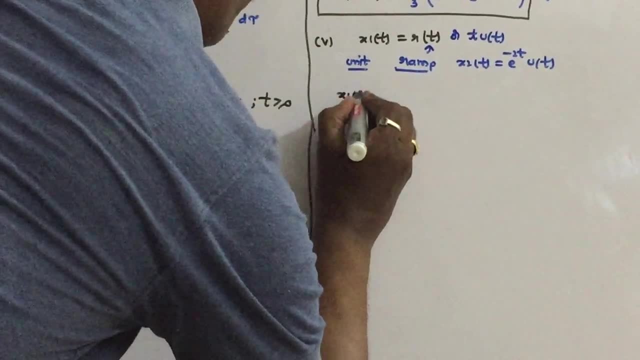 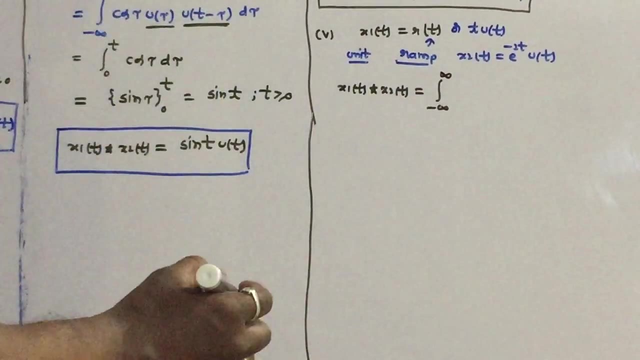 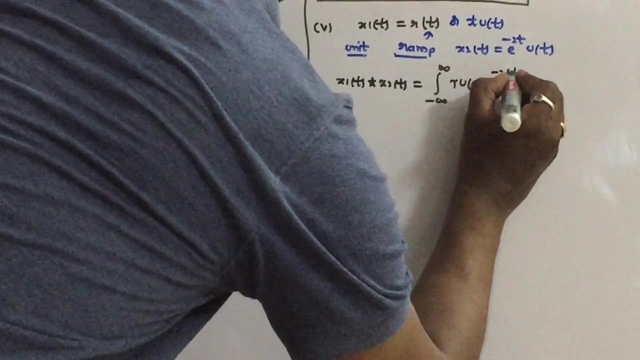 First I will write the formula x1 of t convolution with x2 of t. So that is equal to integral minus infinity to infinity. What is x1 of tau Tau into u of tau. What is x2 of t minus tau e power minus 2 into t minus tau, into u of t, minus tau d tau. 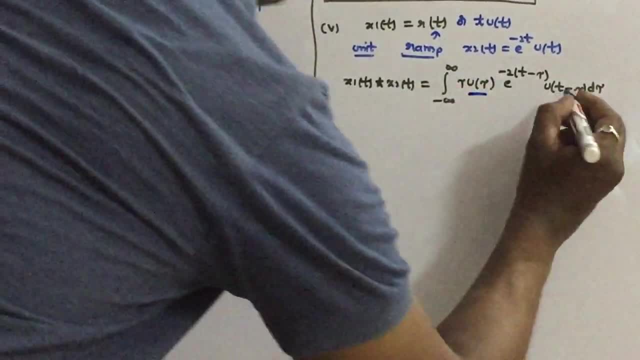 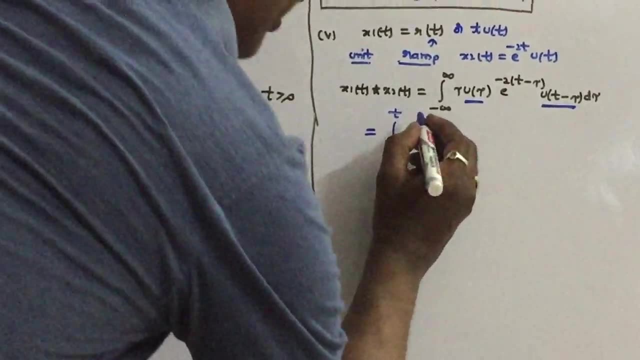 So you can replace because u of tau, u of t minus tau. So just change the limits from 0 to t So you can write it as. so you can write it as from this: integration: e power minus 2t is a constant. 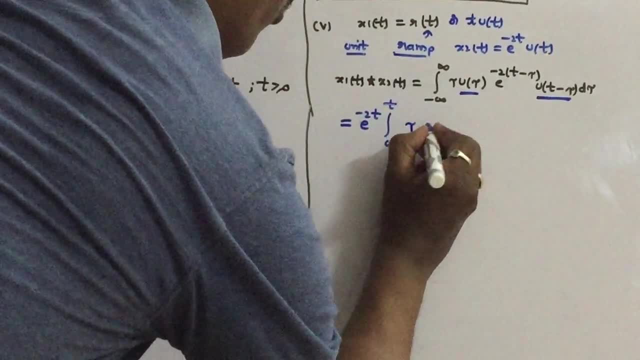 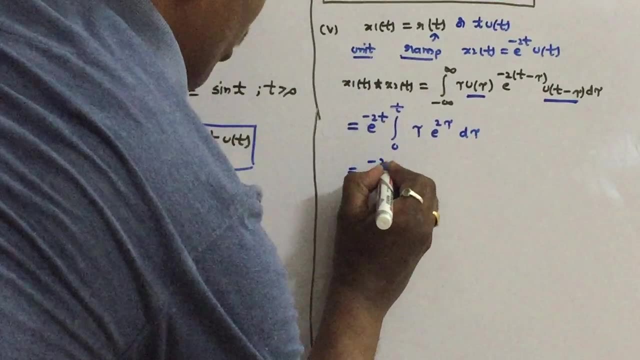 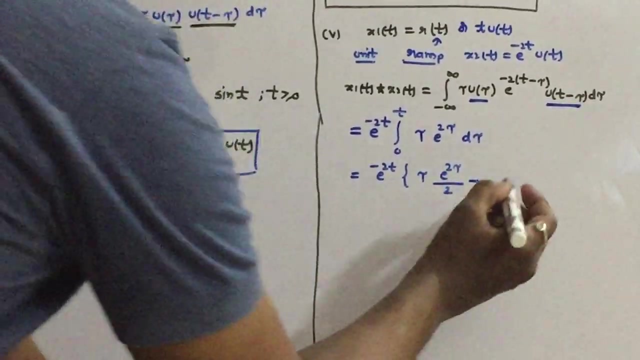 You can write it outside. So this integration will become tau into e power 2, tau d tau. Just apply the UV rule. So e power minus 2t into first function, into integration of second function, is e power 2, tau by 2 minus integration, differentiation of tau is 1.. 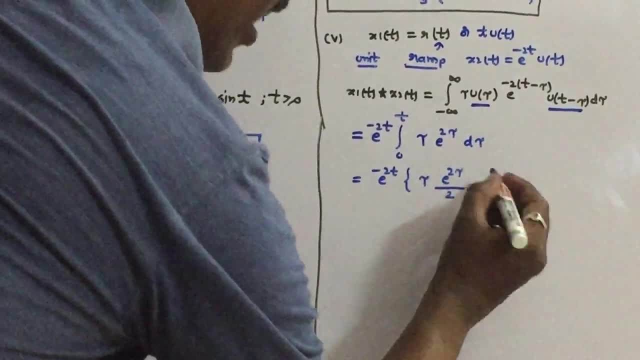 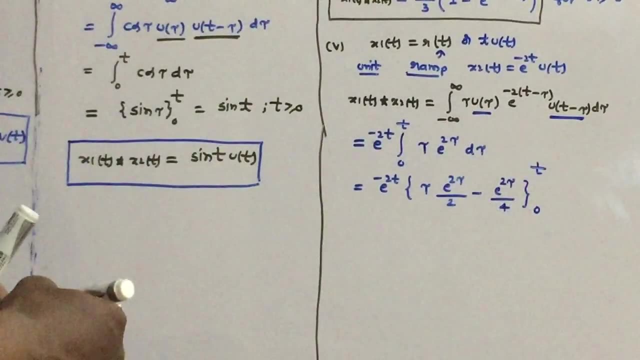 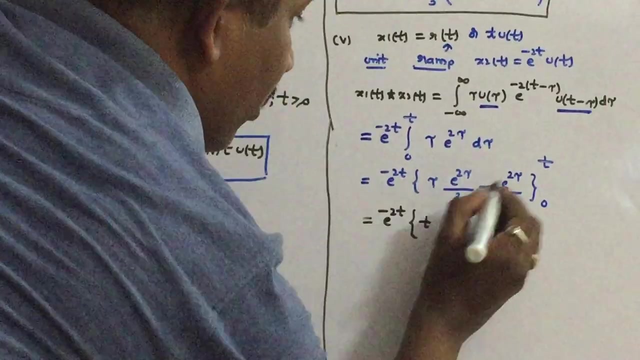 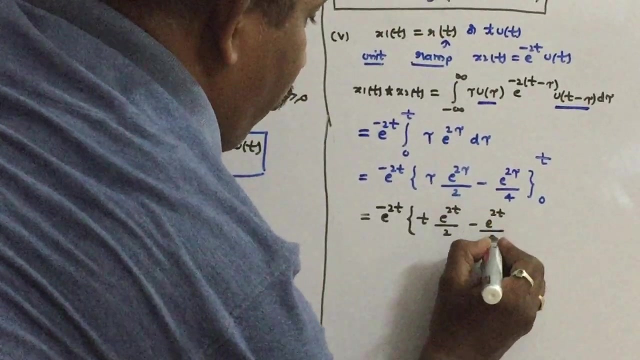 Integration of e power 2 tau is e power 2 tau by 2.. If you again integrate e power 2 tau by 4, will come Substitute the limits 0 to t, So therefore, So e power minus 2t into, so t in place of tau. substitute t. e power 2t by 2, e power minus 2t by 4.. If you substitute in place of tau 0, this term will become 0, plus it will become 1 by 4.. 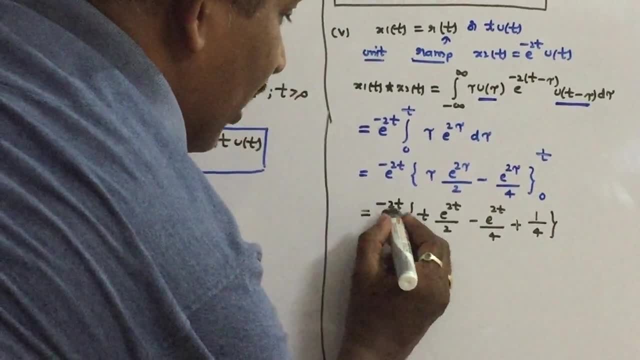 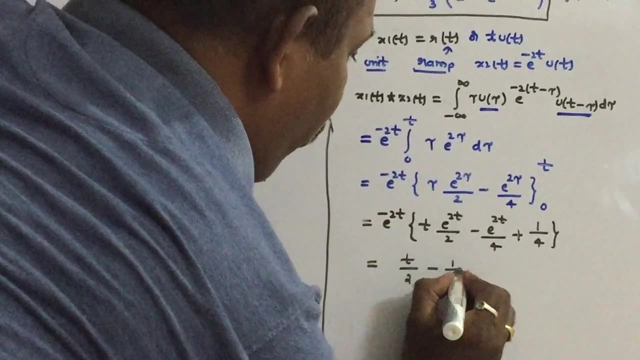 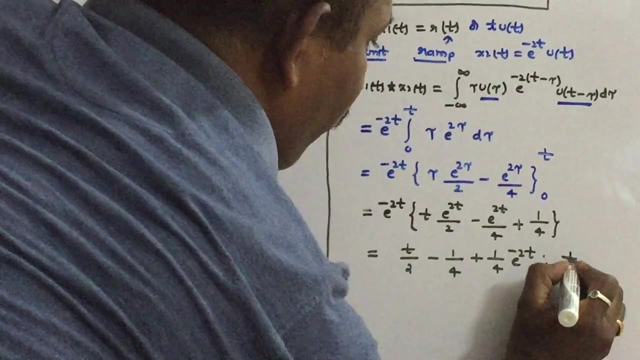 If you multiply, you can see that the first term will come out as t by 2.. The second term will come out as minus 1.. 1 by 4- the last term- we come out as 1 by 4 into e power minus 2t. we have to write for. 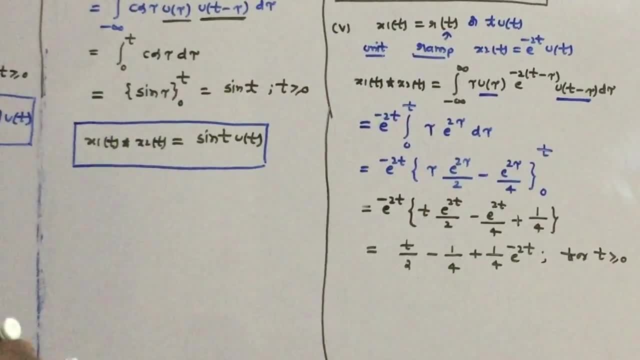 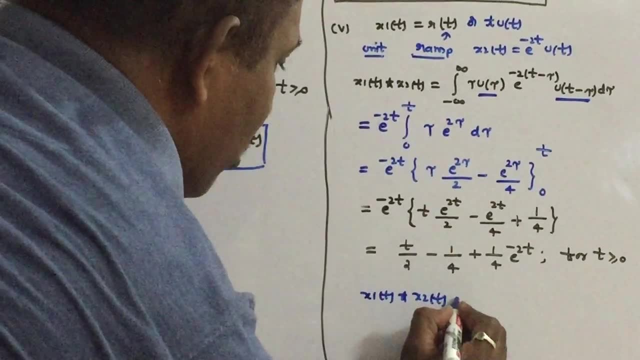 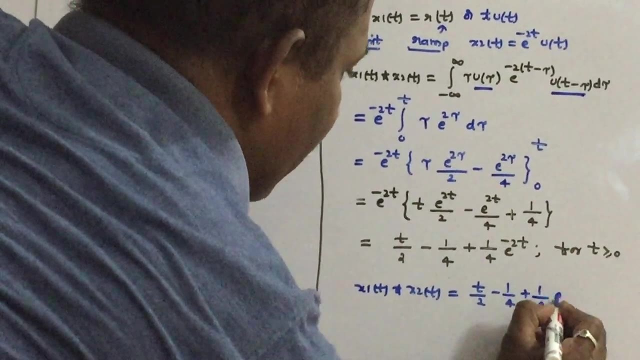 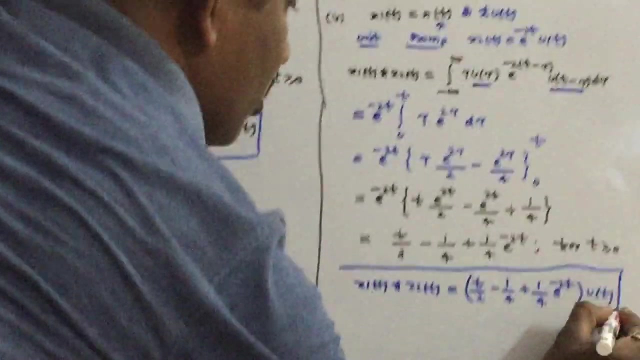 t greater than or equal to 0 or otherwise. we can write the same answer also: x1 of t, convolution with x2 of t. same answer is written as: t by 2 minus 1 by 4 plus 1 by 4 into e power minus 2t into u of t. so this is the answer for this fifth question. so very very. 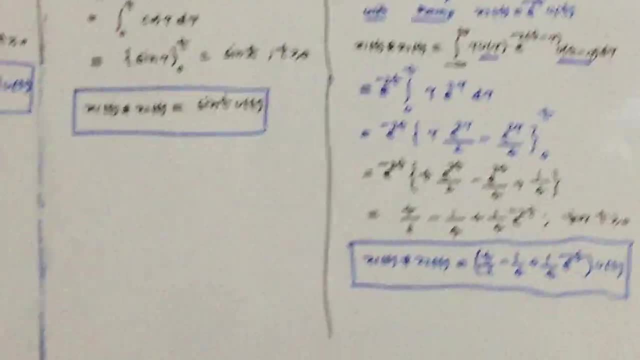 important question in the examination finding convolution of two signals. so this is about this problem, thank you,